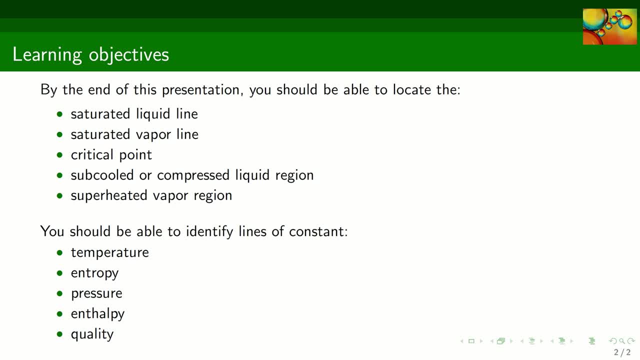 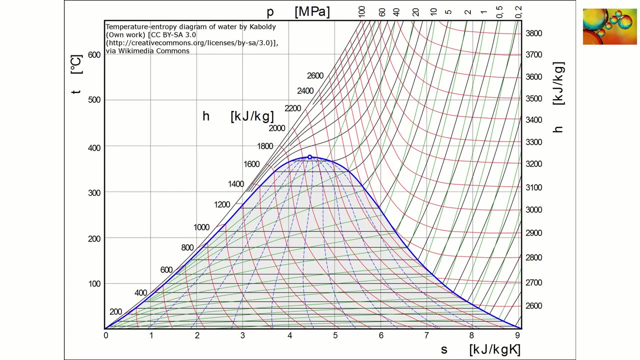 and the superheated vapor region. You should also be able to identify lines of constant temperature, entropy, pressure, enthalpy and quality, which is the vaporized fraction. This is the temperature entropy diagram of water. Observe that the horizontal axis is for the. 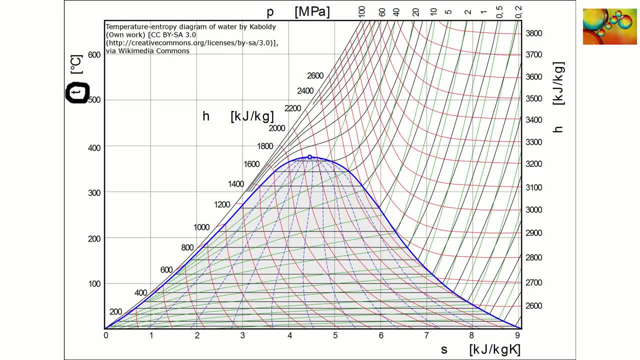 entropy and that the vertical axis is for the temperature. Throughout the presentation we'll use thick black lines to highlight features of the diagram. Here we highlight the saturated liquid line and here we highlight the saturated vapor line. Between them we have a two-phase region. 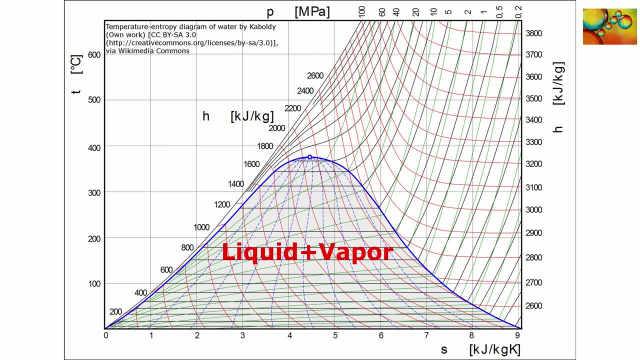 If a system is represented by a point within this region, it will have a liquid phase and a vapor phase. The saturated liquid line and the saturated vapor line come together at the critical point of the pure substance. This is the limiting situation for the coexistence of a liquid and a vapor phase. 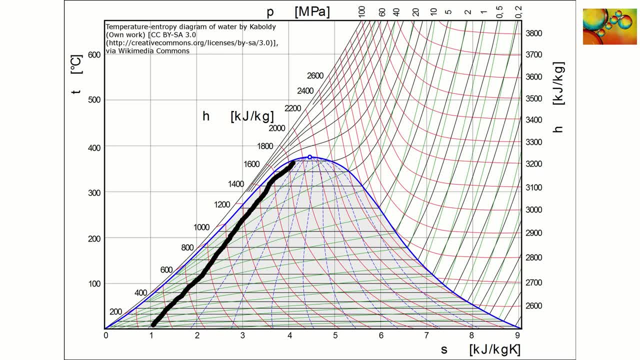 Inside the two-phase region. this diagram shows lines of constant quality. Quality is the ratio of the mass in the vapor phase to the total mass of the system. Close to the saturated liquid line, the quality will be small because there is little vapor in the system, For example. 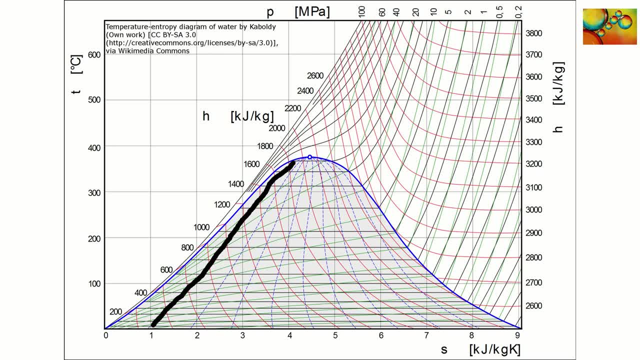 the highlighted line in this slide has quality of 0.1,, meaning that only 10% of the mass is in the vapor phase. The line highlighted in this slide has quality of 50% and the line highlighted in this slide has quality of 90% and observe that it's close to 70%. 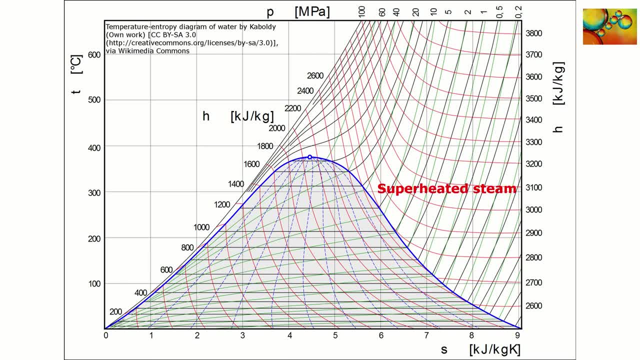 saturated vapor line. to the right of the saturated vapor line we have the superheated steam region. to the left of the saturated liquid line we have the compressed or subcooled liquid region. but bear in mind, if you move too much to the left, you may end up in the solid region which is not shown in detail in 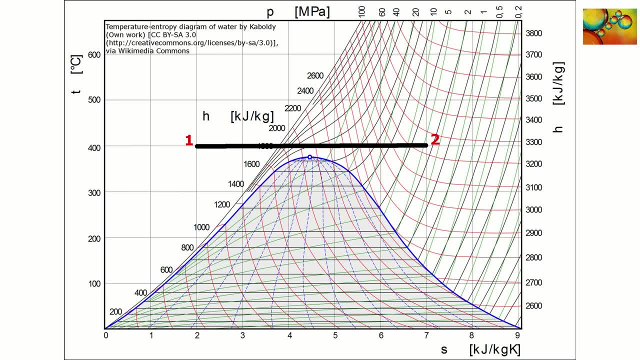 this diagram, an isothermal process is represented by a horizontal line. for example, a process that starts in state 1 and proceeds horizontally to state 2 happens at the constant temperature of 400 degrees Celsius. an isentropic process is represented by a vertical line, like the one shown in these slides. an example: 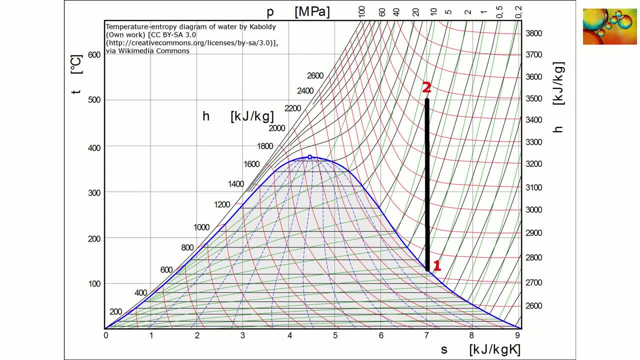 would be an adiabatic and reversible compression, starting from state 1 and taking the system to state 2. this slide shows an isobaric three-state process that starts from point one, in the superheated steam region, and then goes to point two, which is a saturated vapor, and onwards to state three, which is a 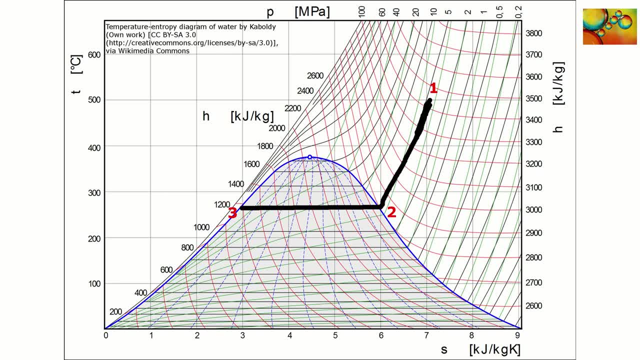 saturated liquid. observe that between states two and three not only the pressure remains constant but also the temperature, because the line connecting points two and three is horizontal, and we know that the horizontal line in this diagram represents an isothermal process. therefore, between points two and three the process is at the same time isobaric and isothermal. here the process 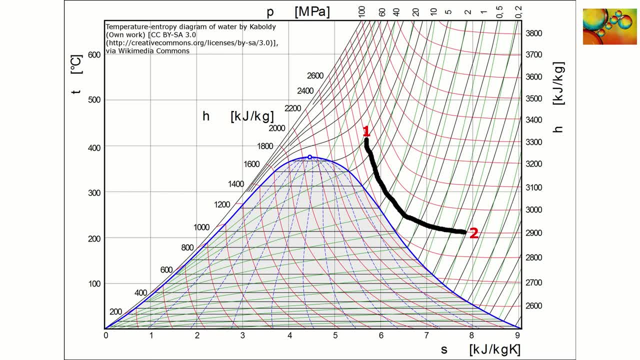 that happens between states one and two occurs at constant enthalpy. it's called an isenthalpic process. an example of isenthalpic process is the expansion of a fluid through a perfectly insulated valve. in addition to the lines we discussed here, there are light green lines. 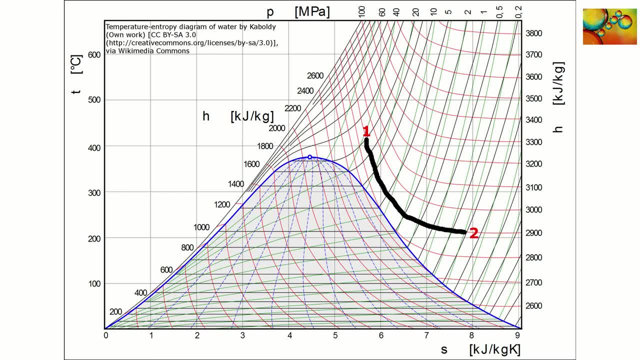 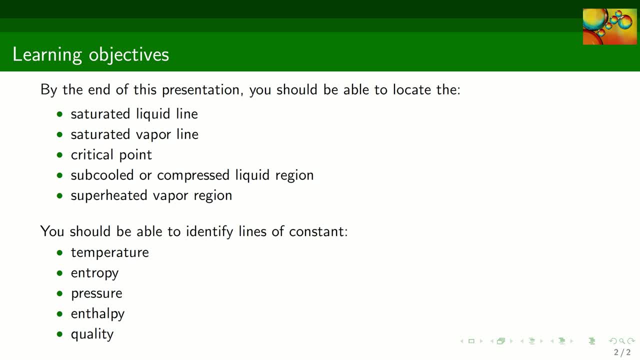 in this diagram and there are lines of constant specific volume. in summary, if you know how to navigate the many lines that the temperature entropy diagram displays, you can represent different types of processes. it's a very rich source of information. thank you very much for watching this presentation. make sure you subscribe.